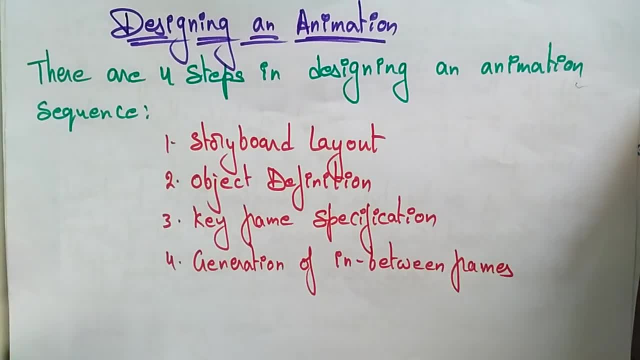 students, welcome back. let's continue with the animations. uh, in the computer graphics. now let's see what: how to design an animations. okay, designing an animation. there are four steps in designing an animation sequence. if you want to make any movement in the picture, in an object, you requires these four steps. so what are those? first is a storyboard layout. next, object definition. 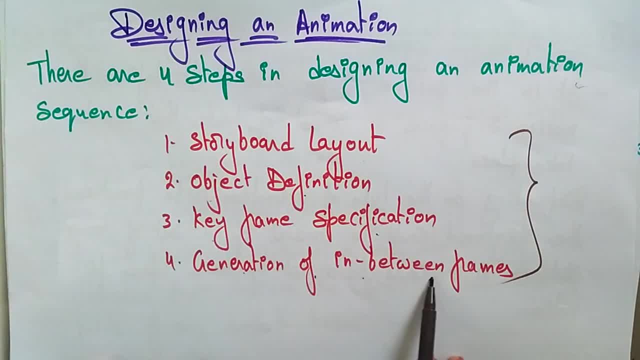 keyframe specification, generation of in between frames. so if you clearly read twice or thrice in these words only you will get the clear idea. so what exactly it's saying? if you want to design any animation, you require these four steps first. they are saying storyboard layout. so suppose if 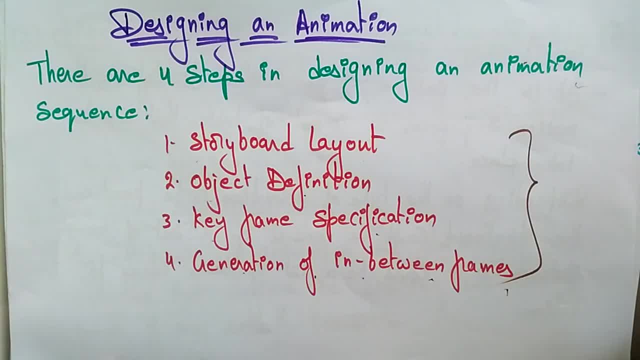 you want to start any movie or if you want to start any animation, what exactly you want first required what you're going to be do. that you have to be written in a pictures. okay, it's just a rough diagram. you need it, okay. so after storyboard layout: the object definitions means in that what I have. 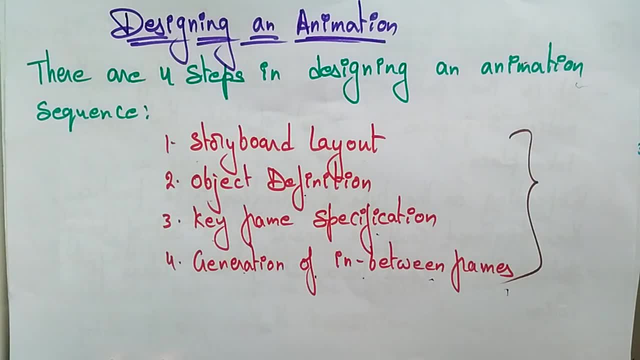 to be included. the different objects, I can include it. if you want to make any a small, let's take a small bit of animation. so in that, if you want to add any objects, okay, so that object definitions you need to be known. next, keyframe specifications. so what is the starting point and what is the ending point? the keyframes, so the story. 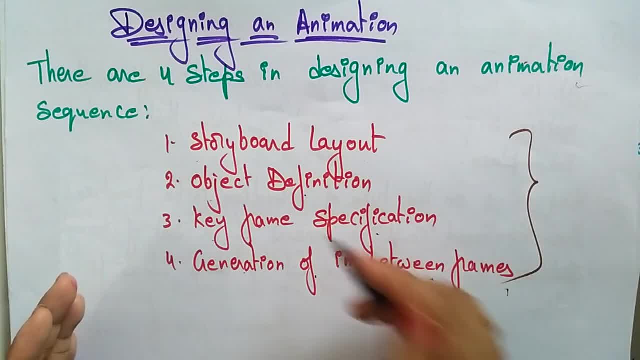 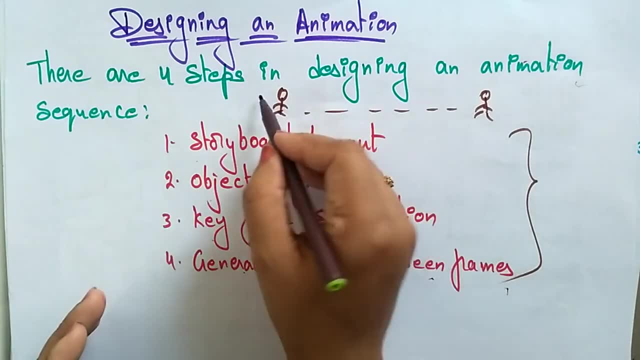 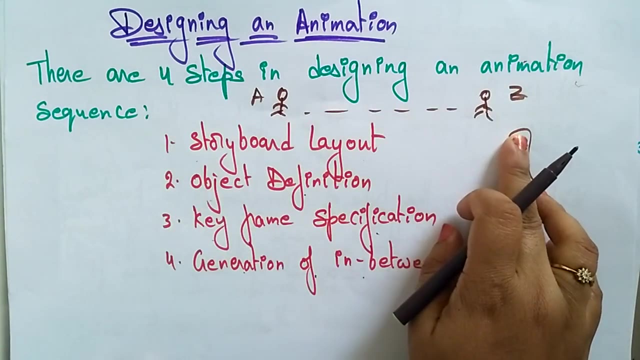 has to be start here and it has to be end like this: suppose the person is walking the same way. okay, he has to move from starting position somewhere in a and he has to move to the z place. from a to z he has to move. so that is a keyframe specification. so in between, how you're going to. 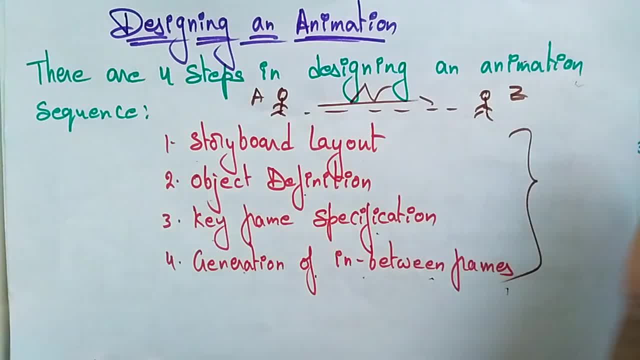 move. it's a straight line or up and down. it's a straight line or up and down. it's a straight line down, or from down to up, like the. whatever it may be, that is a generation in between the frames. okay, first storyboard layout. what is the storyboard layout I'm writing here? this person wants to reach. 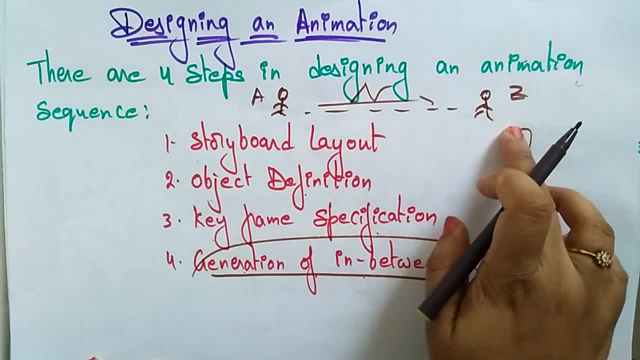 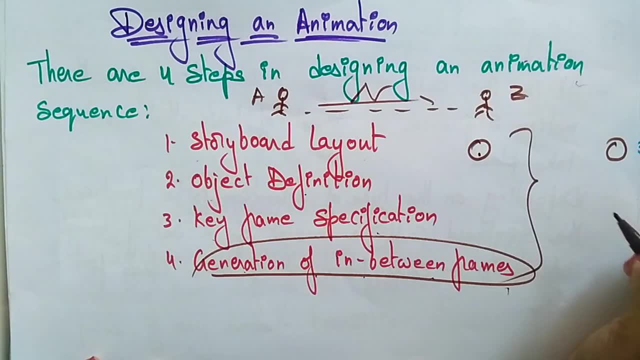 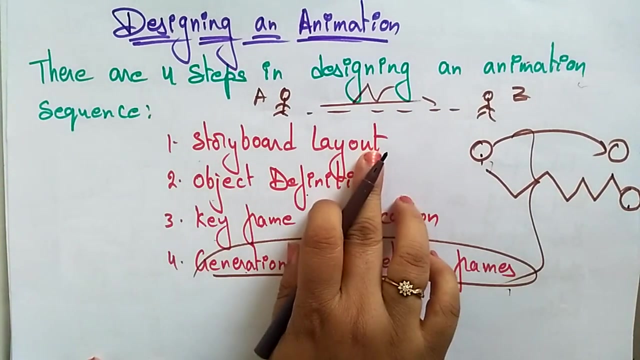 to z place. so this is an object. this object has to move to the z place, so just takes the ball. okay, this ball I'm throwing and another person is going to be catch. okay, so this ball I'm throwing, just throwing. okay, or I'm just bouncing, I'm bouncing the ball, so this ball I'm bouncing. so first the story layout. 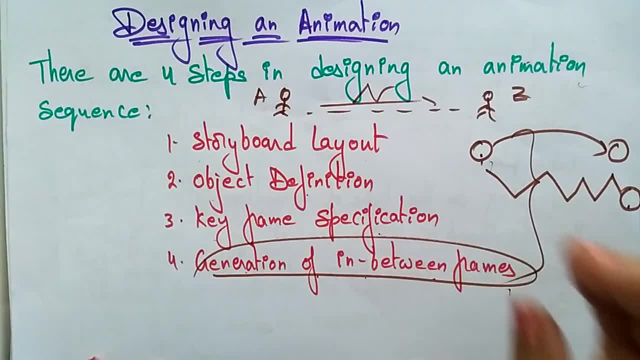 what I'm taking. so here, the ball has to be there, the ball has to be bounced like this. so, first step, second step, third step. first step, second step, third step, fourth step, finally, it reaches. so that is a storyboard layout. next, I'm including the object definition. what object, so what type? 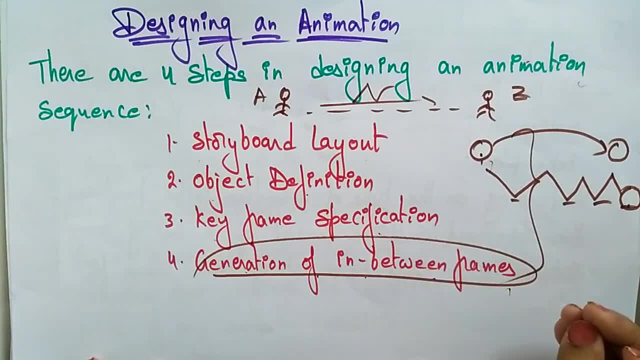 of ball I'm using. okay as it. what type of color it is I'm using? there is a whole storyboard layout. object definition: next is a keyframe specification. so how much, from where i am starting and where i am ending. next, generations in between frames. so this is the generation between frames. so how? 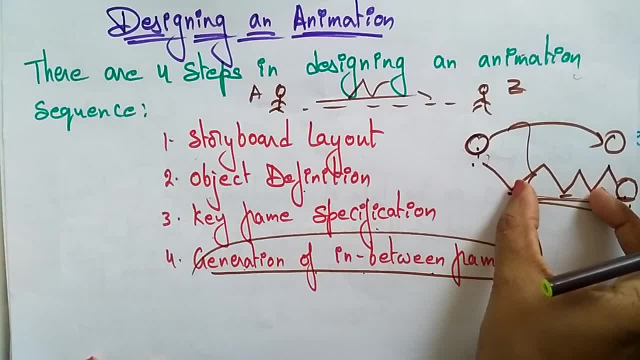 the ball is going to be bounce. so this, everything will be done by the computer. okay, the thing is you have to do the storyboard layout and you have to give the object definitions and the keyframe specifications and bouncing everything will be given by this. in between frames will automatically. 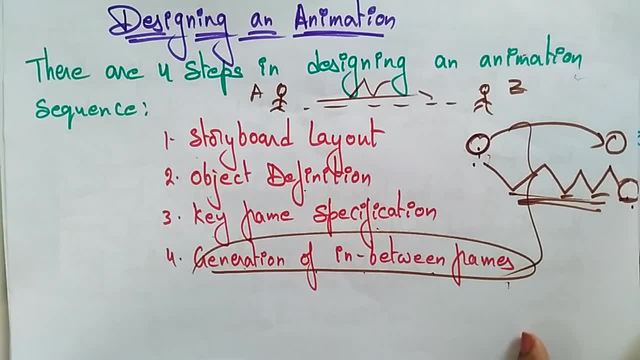 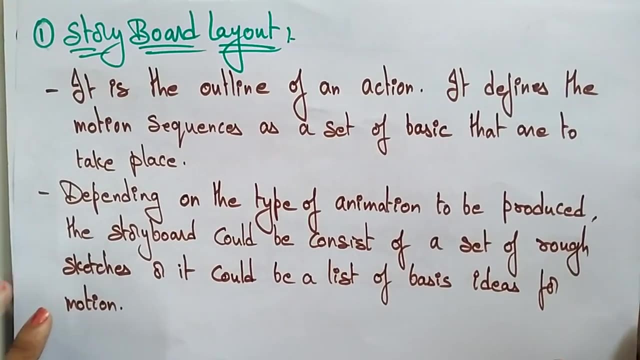 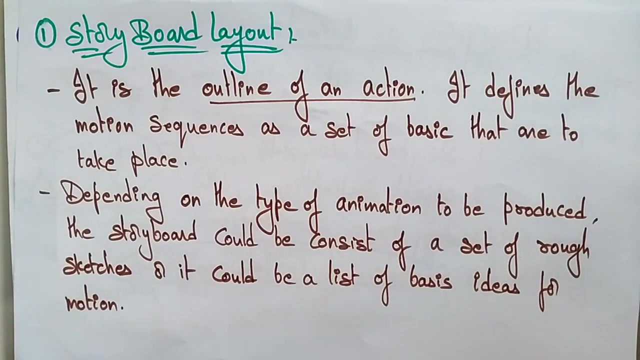 generated by the computer. so this is an overview of this designing and animations. you require this. four steps: first, storyboard layout: object definition, keyframe specification, generations in between frames. now let's see, one by one, a storyboard layout. okay, so it's just an outline of an action. so what i said? what do you want? exactly that you have to be right in the paper. 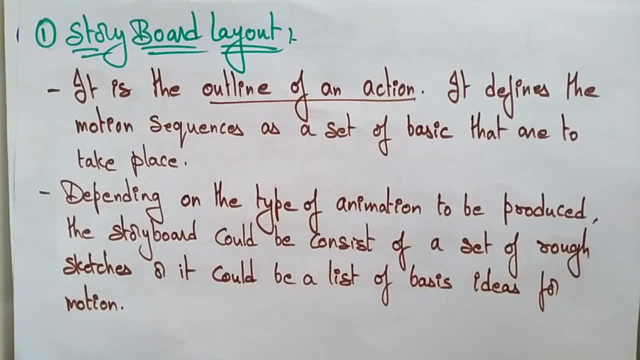 just like a uh. if you take the software engineering, if you want to develop any product, what you are going to do your first, you need the requirements. that is a storyboard layout. you need the requirements and you have to just imagine: this is the input and this is the output. okay, 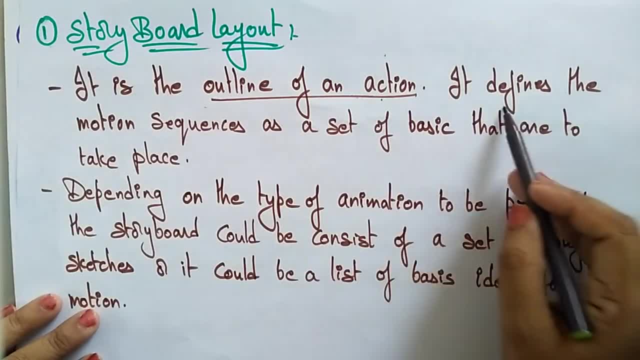 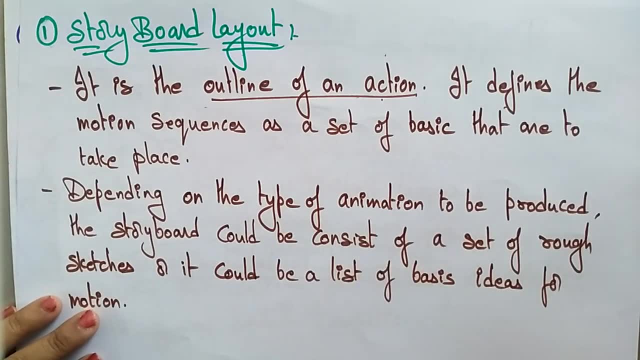 so that is a storyboard layout. it's an outline of an action. it defines the motion sequence as a set of basic that ought to takes place. so, depending on the type of animation- so this, remember that- what type of animation you are using: the cell animation or kinematics animation or computer? 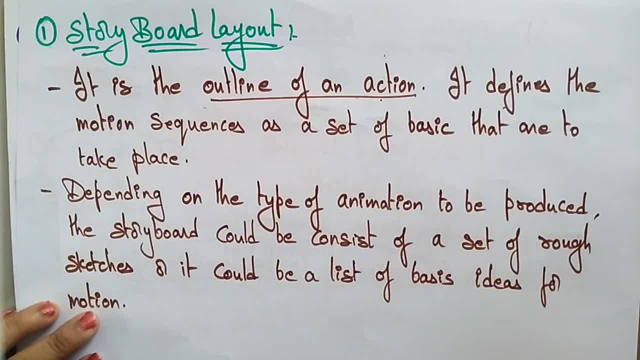 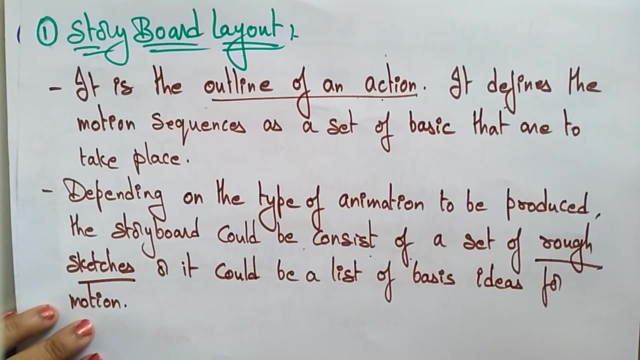 animation or morphing. so what type of animation you are using, that should be dependent it's depending on the type of animation to be produced. the storyboard could be consist of set of rough sketches. so, starting what you needed, you need a set of rough sketches. okay, how the bounce is ball. 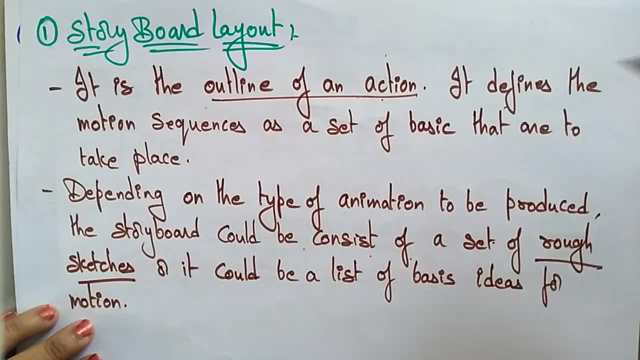 starting. it takes one step, another step, another step. so like that it's a rough sketch you need. you have to be prepared, or it could be a list of idea livro, but you have to be prepared, or it could be the first idea. it is a basic idea, rubic. 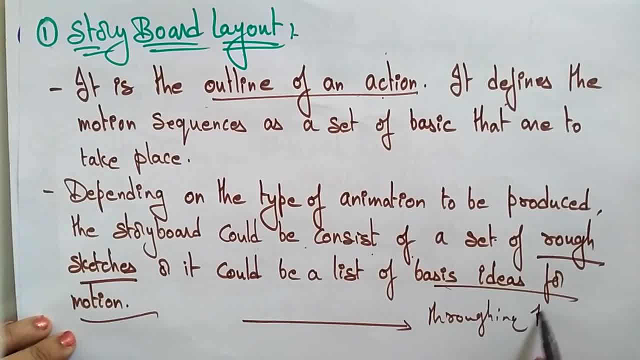 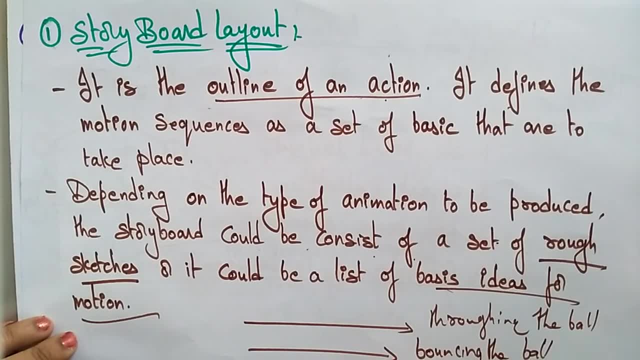 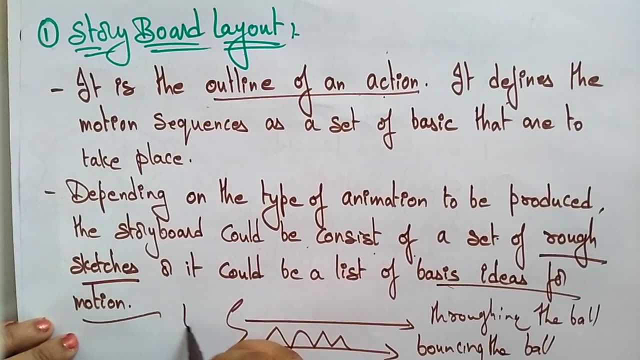 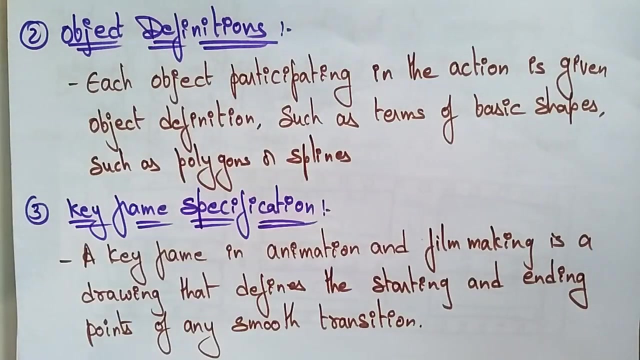 I and the basic idea motion and basic ideas of a motion, so how it is going. okay, are you throwing the ball? throwing the ball okay, or you bouncing the ball? okay, or you bouncing the ball, so that you have to be decide. that is a storyboard. they are the basic idea motion. the basic idea motion. 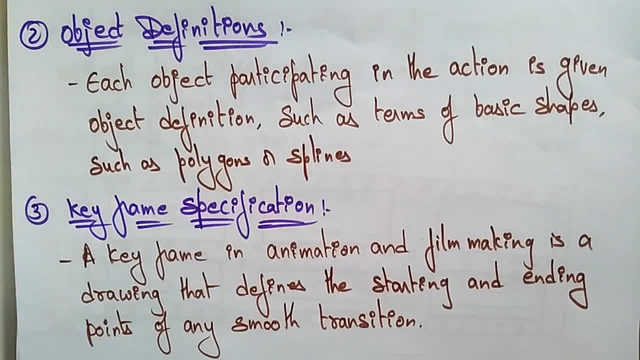 okay is the object definition. so after that, what you have to take, you have to decide what type of objects that you are using. each object participating in the action is given object definition, such as terms of basic shapes, such as polygons or splines. so, whatever i said- okay, here i'm taking a ball- is: 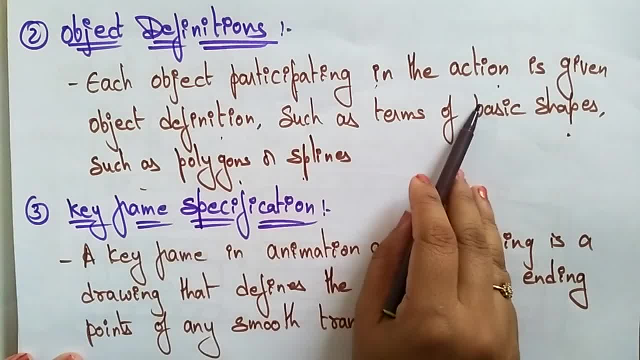 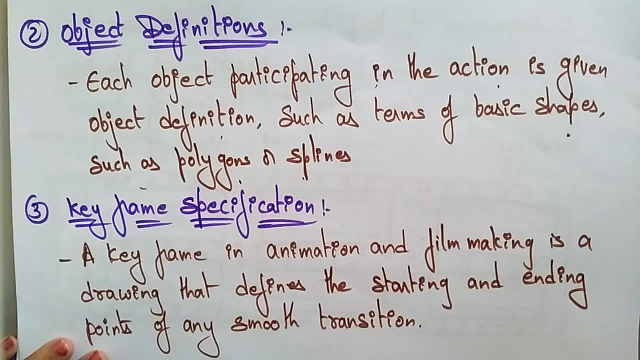 bouncing animation. so here the object participating in the action is given by object definition. so what definition i'm giving, what term terms of basic shapes i'm using, whether i'm using the round ball, okay, or just i'm using some square. it's a, it's just a stuff, or i'm using a polygon. 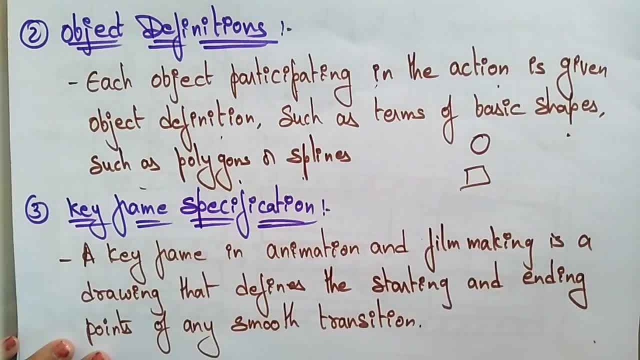 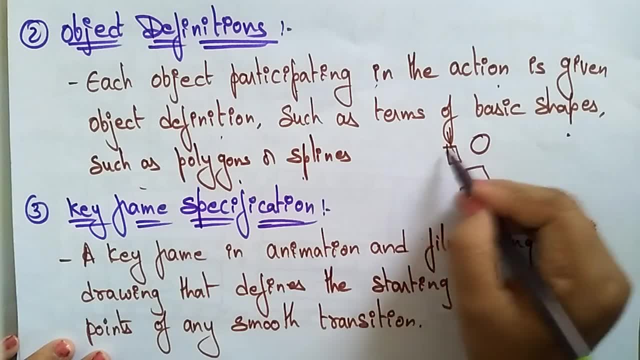 and what type of material i'm using. that is the object definition. so in between this i'm using anything, okay, or i'm using the bat or not. this is another object. so that specific definition also you need to be give. so i'm kicking with the bat or are you kicking with the shuttle rocket or 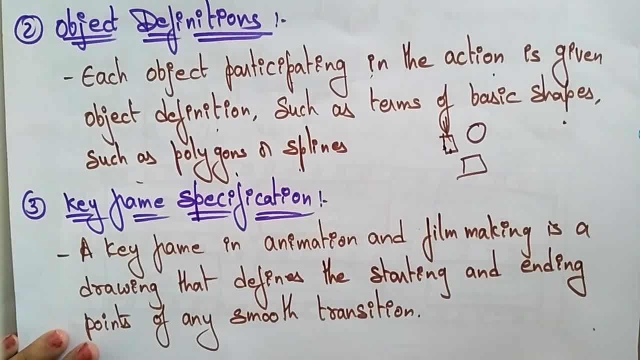 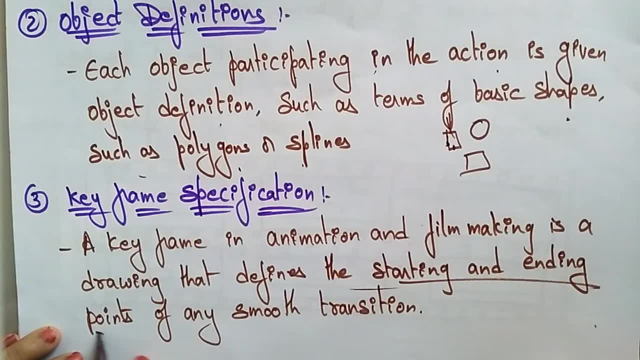 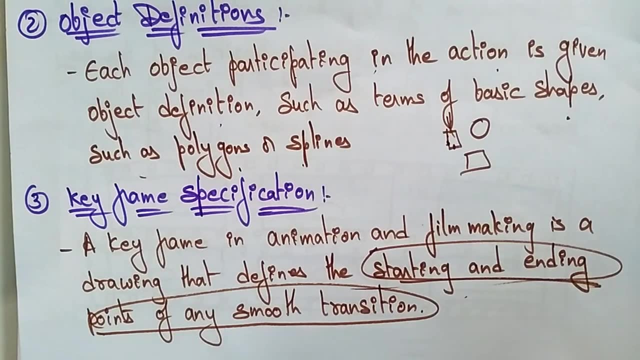 whatever it means, uh, that you need to be give next sequence: keyframe specification. a keyframe is an animation and film making is drawing. that defines the starting and ending points of a smooth transaction. so this is remember that a keyframe specification is the starting and ending points. 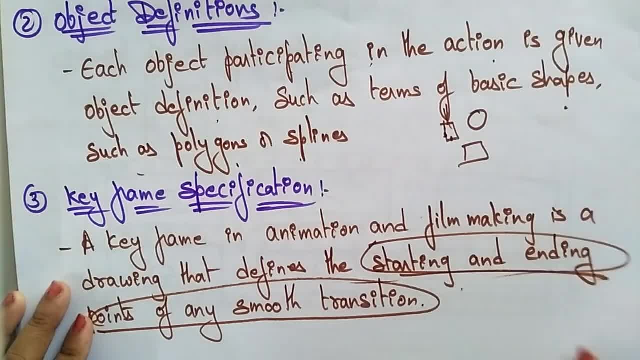 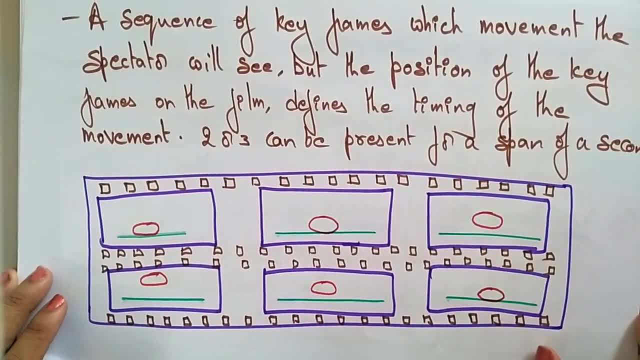 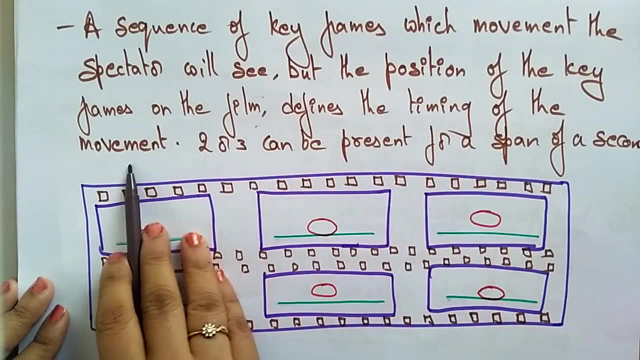 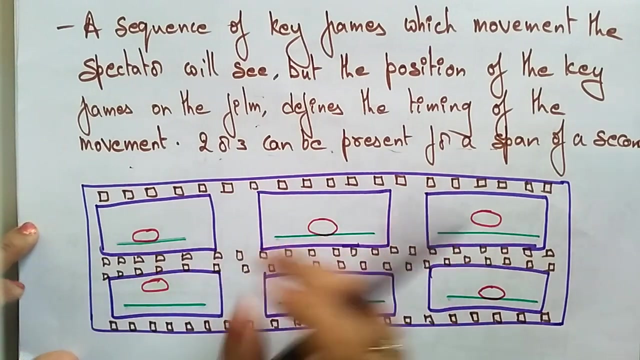 of any smooth transitions. you call it as a keyframe. okay, now let's see the keyframes. a sequence of keyframes with moment the spectator will see. but the position of the keyframes on the film defines the timing of the moment. two or three can be represented for a span of a second. so let's take this is a film. okay, these are the frames. 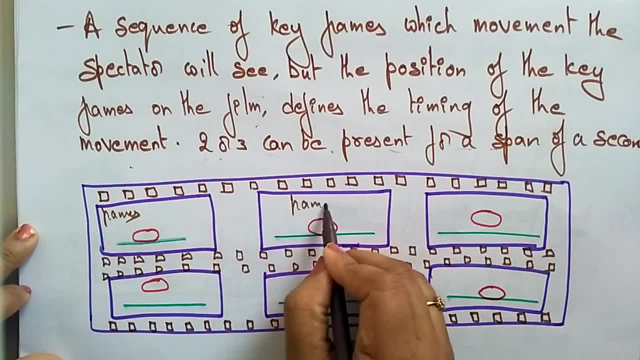 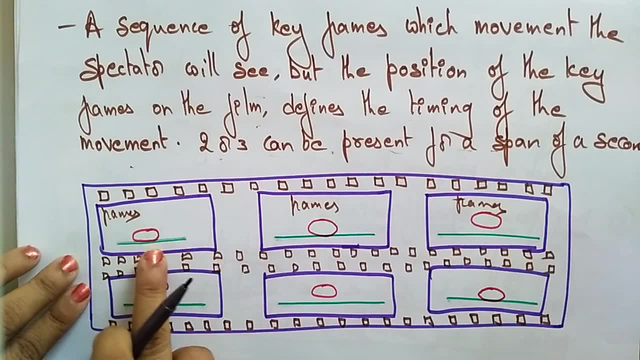 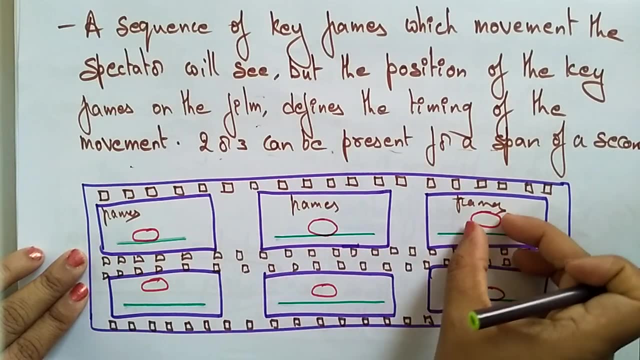 okay, these are the different frames, so this is a starting, the starting frame. i'm just a ball, is there? so uh, means one image is there. that image is growing up. okay, next it is going up, up and coming down and placing down. so just a moment is observed here, starting and ending. 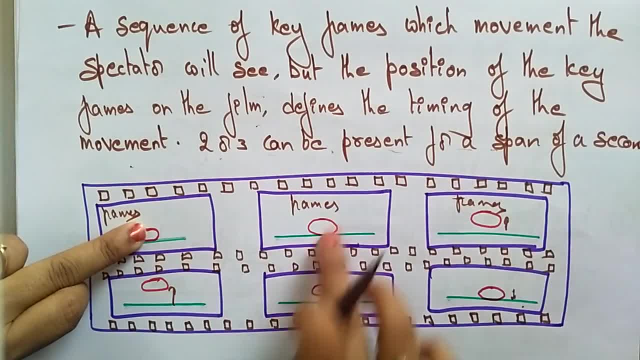 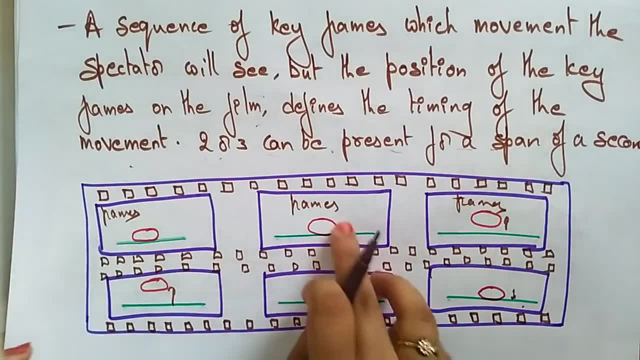 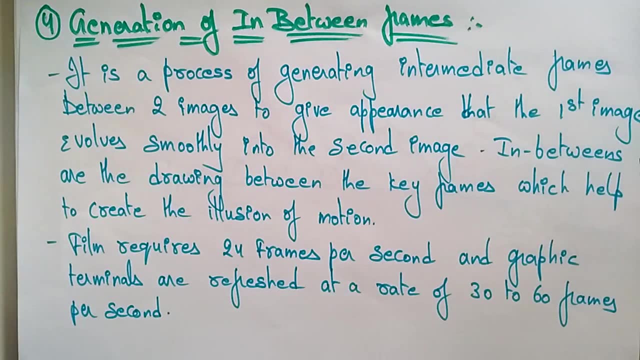 frames, so in between that some actions are performed. this is an animation. this is an animation, okay, so you call it also. so in between frames also, you can call these as an in between frames also. and the next type of next, next sequence in the animation is the generation of in between frames. 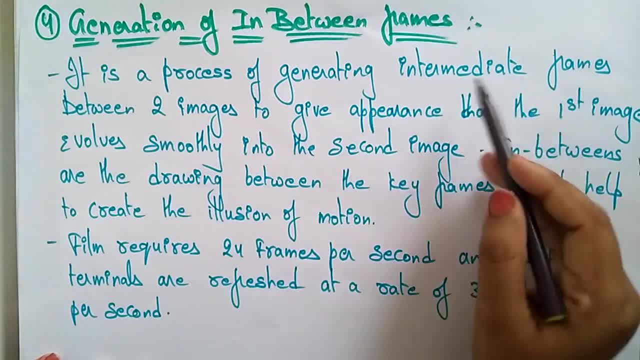 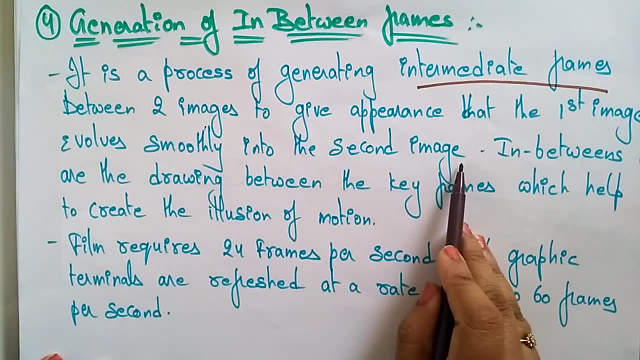 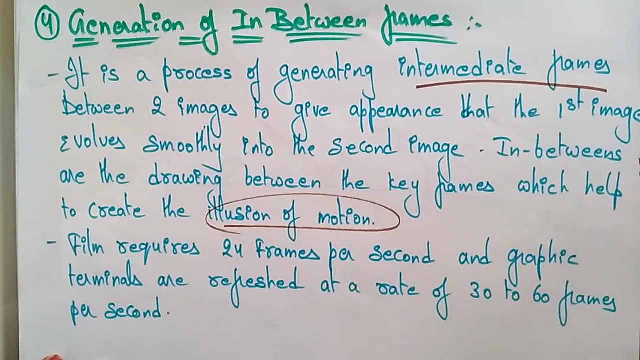 so it is a process of generating intermediate frames between two images to give appearance that the first image evolves smoothly into the second image in between frames, or drawing between the keyframes, which helps to create the illusion of motion. so, whatever i said, if you are bouncing a ball, the starting first image and the second image is evolving smoothly into the second image. 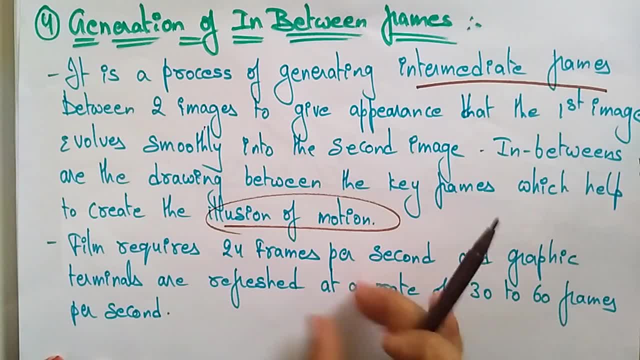 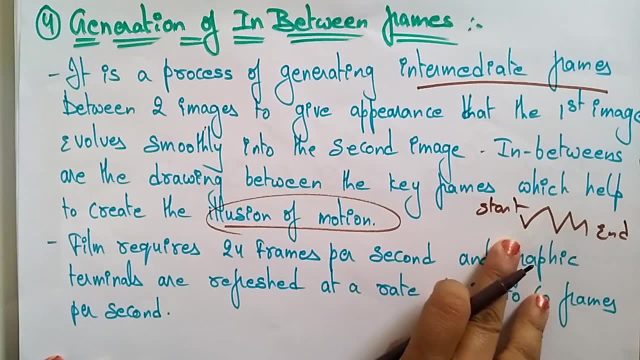 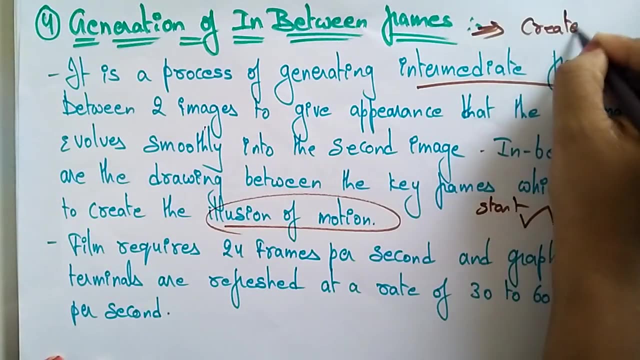 okay, so in between the keyframes, that is a start- and and in between so many frames are there, that is a frames which creates an illusion. so exactly what it taking in between frames creates illusion. okay, i hope you clearly understand what exactly the in between frames, in between frames are. 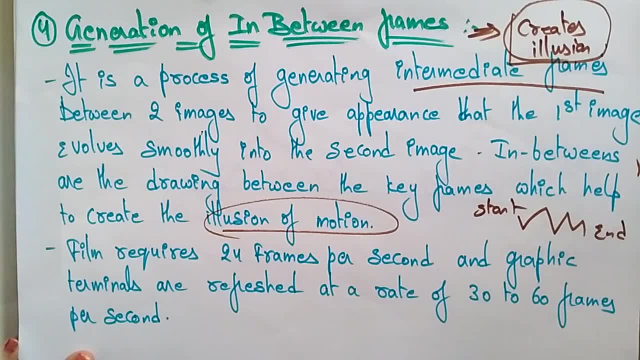 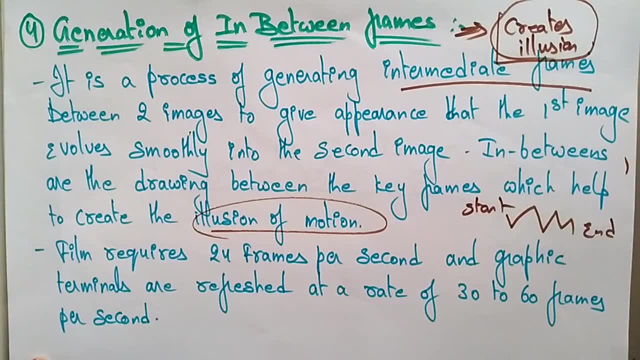 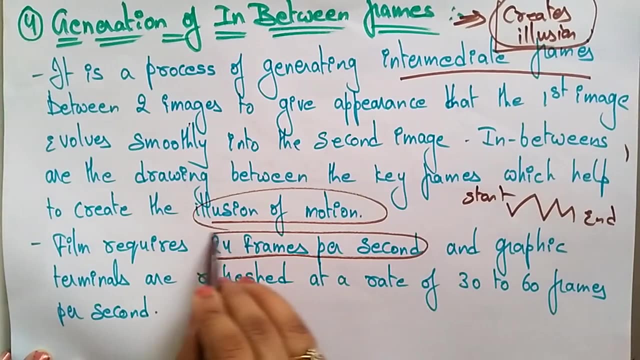 creating illusion and the three keyframes, or whatever you are able to see. that is start and end, that is a keyframe and in between frames or the create that is going to be create an animation, that is an illusion of motion. a film requires 24 frames per second approximately. if a film requires